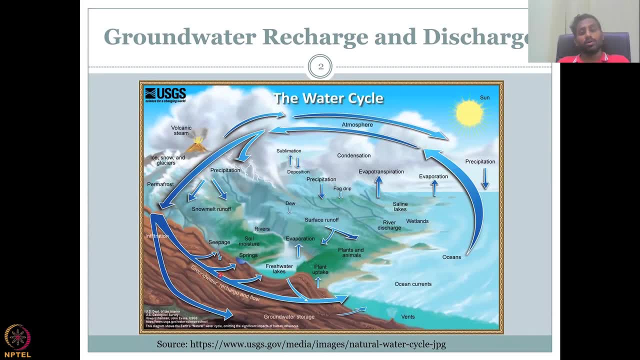 and how groundwater comes out, in terms of natural, which is seepage into the freshwater, lakes, springs, etc. And also to the oceans, are called groundwater discharge. Now, because of recharge, they can also be discharged. Same: because of discharge, they can be recharged. 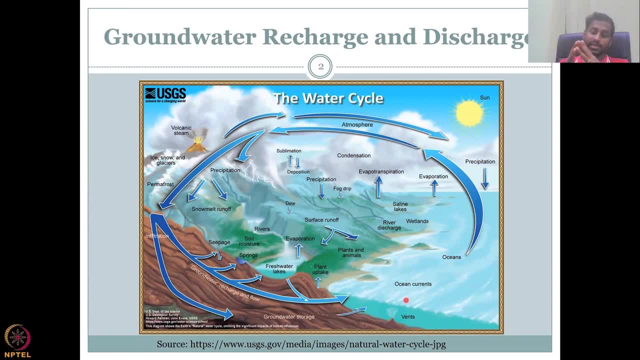 We will come back to that in the next lecture, Thank you. So let's move on into how these two components are interlinked. Also, there is a human component, or anthropogenic. We do have groundwater recharge because of augmented recharge, induced recharge. 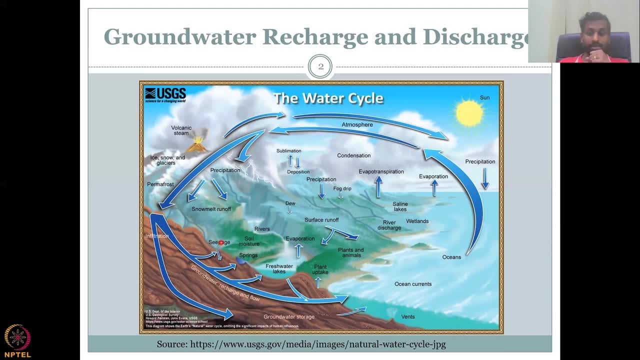 etc. On the other hand, there is groundwater discharge through human actions, Most importantly when you pump out. So in this week's lecture we will look at the key parts in which groundwater recharge and discharge happens. More importantly, we will look into methods to quantify groundwater recharge and discharge. 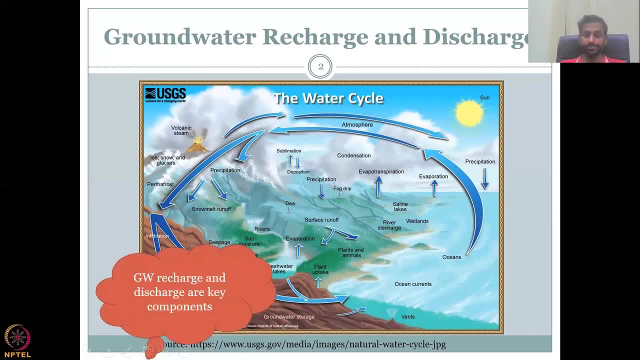 In the first class of this week, we'll also look at how groundwater recharge and discharge forms key components in the hydrological cycle. If you look at the cycle here, for example, if groundwater recharge doesn't happen or discharge doesn't happen, what do you think will happen is that this water will never. 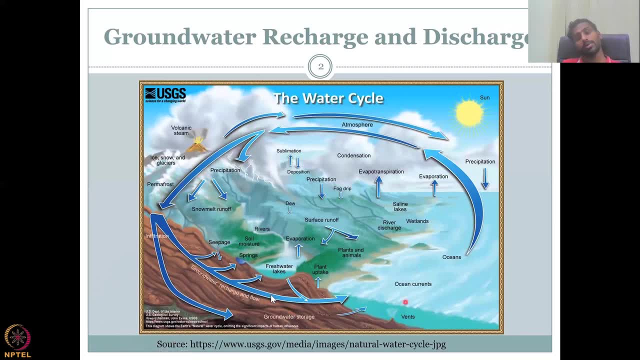 get into the aquifers, nor it gets out as base flow. So the cycle would be more faster, because every water that falls on the ground would either be stored on top as lakes and rivers, So when it runs off back into the ocean, whereas the groundwater recharge actually delays the 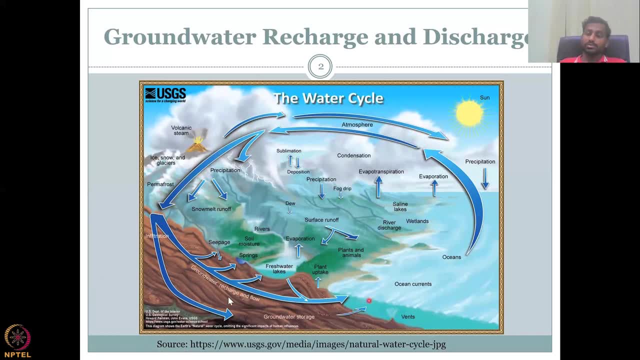 water in completing the cycle. These are much, much faster time steps compared to the groundwater movement. So basically, your water goes through a slower cycle and it takes some time for recharge and discharge. If you look at here clearly, when groundwater is coming into this phase, for example at 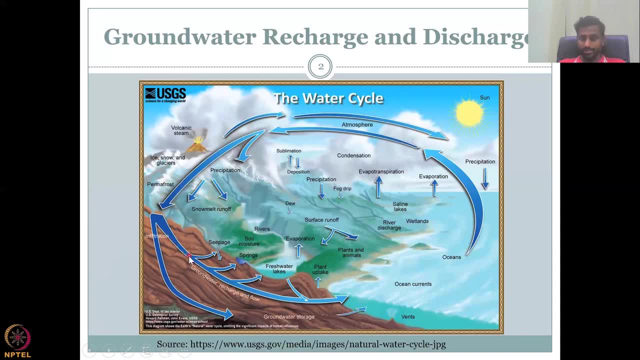 this particular location, groundwater is recharging And if it is taking this path to go out, it is discharging. But in between, like for example this point, groundwater is recharging right Because water is flowing through it, recharges. 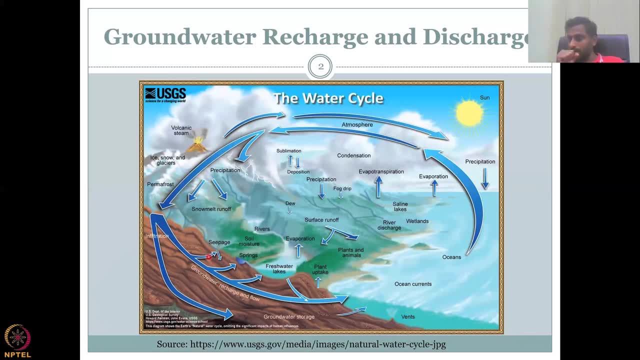 It doesn't stay long, but then it discharges out. So this is where the connections happen, But more importantly, on this water cycle that we used to see a lot of these hydrological components. groundwater is a key component without which most of these cycles would not. 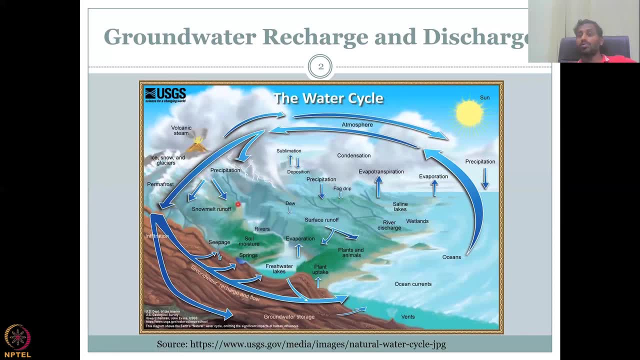 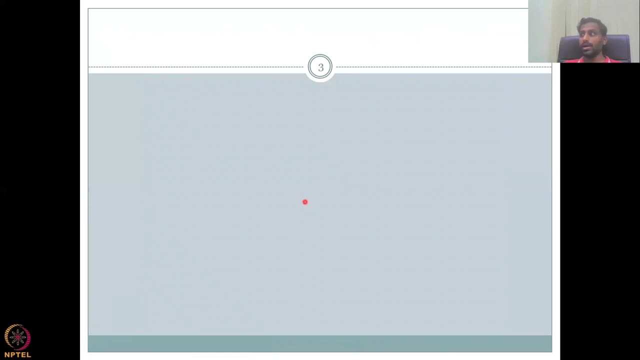 complete itself and or it will be more flashy- flashy as in quicker. So that is why I'm again saying that groundwater recharge and discharge are key components in the hydrological cycle. Let's look at what forms the basis from the hydrological cycle. 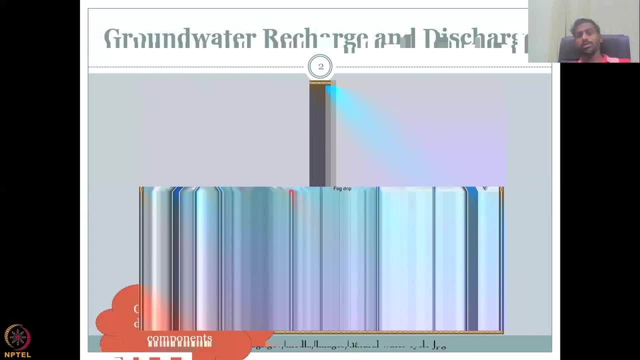 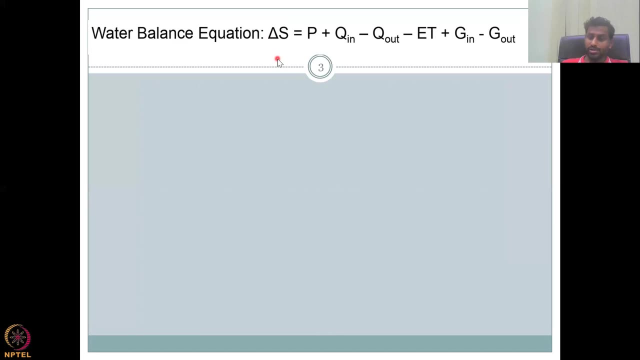 Yes, the water balance equation. How is groundwater defined here? our road recharge and discharge, So your del S in your hydrological cycle is the net storage in the basin. Okay, let me draw a quick basin for you, or an area. So this is your area. 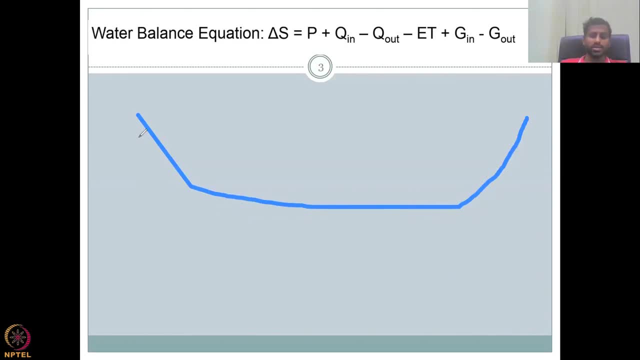 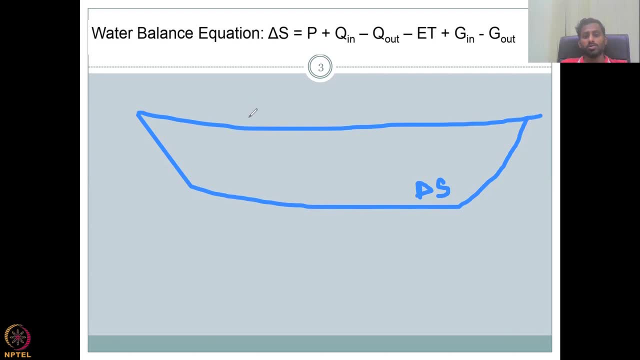 Del S. Precipitation is what comes in. P, Q in is what comes in as surface water, Q out is what goes as surface water. ET is loss, So it goes out. Okay, All the minuses are going out, So this is ET loss. 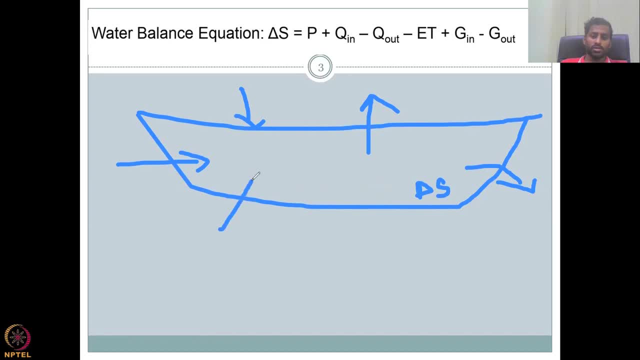 This is your Q out, and then you have your groundwater in, which is from the basement. I am saying, okay, this is groundwater coming in and groundwater coming out. So I will explain all these terms in the hydrological cycle. However, for our this week lecture, these two components are very important. 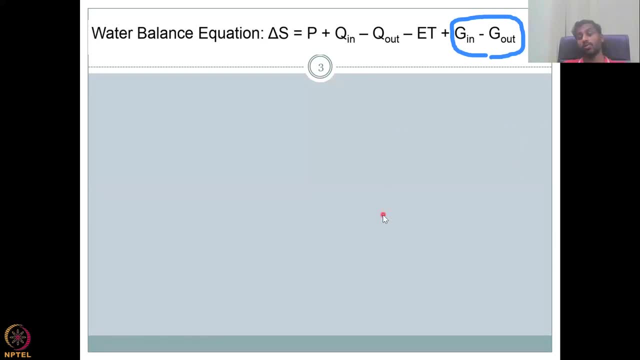 because they define what is g in as groundwater, in, which is your recharge, and g out is the groundwater discharge coming out. So for a system you have in the hydrological cycle, in the water balance equation, a groundwater coming in which is called recharge, because this is your system and 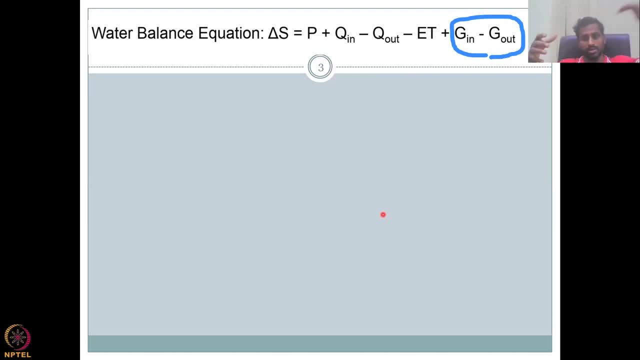 groundwater is coming in, actually comes from bottom, but you can also show that just as a vector it is moving in. Then you have groundwater out, which is you are taking out. Groundwater out can be from the bottom as groundwater seepage or pumps you take out. So del S is change in water. 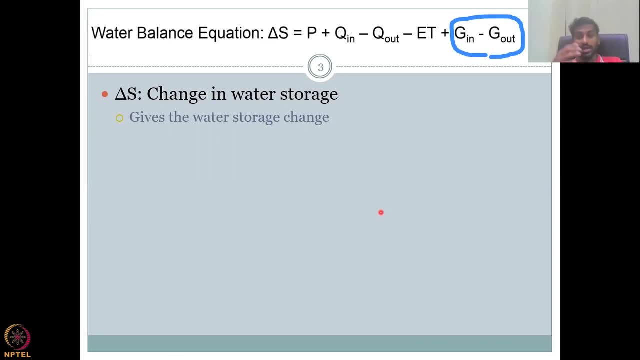 gives the total net water storage. It is the change in any of these components. You can have storage inside your basin by ways of soil, moisture, surface storage or groundwater storage. G in is groundwater in. Groundwater recharge to the system can also be from different basins. So 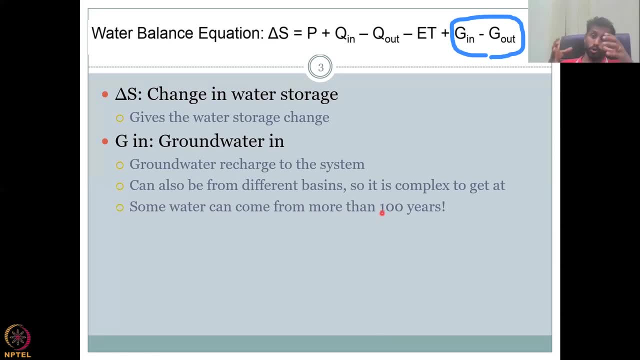 it is complex to get that, which means it is not only from your hydrological basin, it could be from a different aquifer, different basin, because it moves under the basin. So on the top rainfall cannot come from other basin to inside unless it is coming as q in. So please understand that g in. 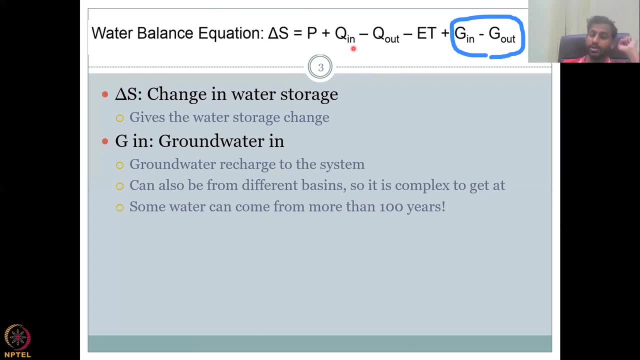 is a very complicated parameter. It cannot be just estimated using your basin boundary. Some water can come from more than 100 years. slash kilometers. 100 years means it took 100 years to travel, So think about how far it should have traveled without. 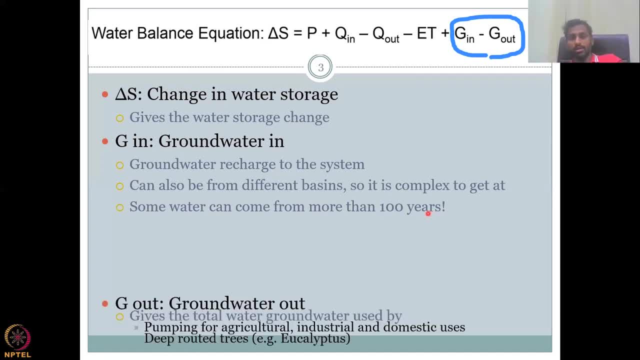 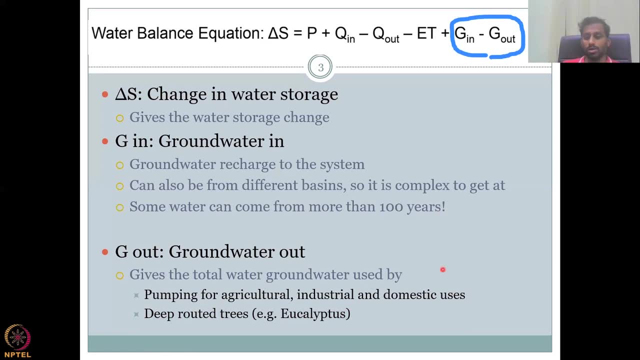 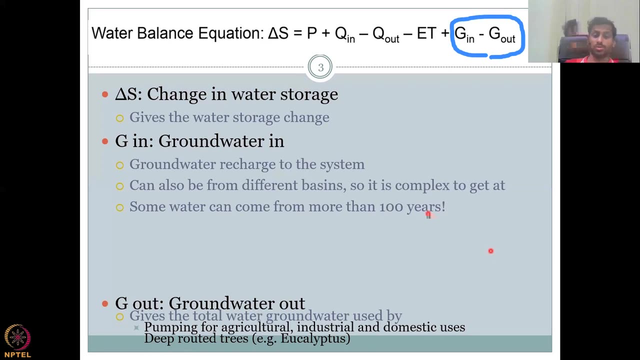 all these disturbances and get into the system. So that is your groundwater in which, in this class, we will be looking as recharge Groundwater out is the total water of groundwater used by pumping for agriculture In the structure of the system. it is the total water used by pumping for agriculture In the structure of the system. it is the total water used by pumping for agriculture In the structure of the system. 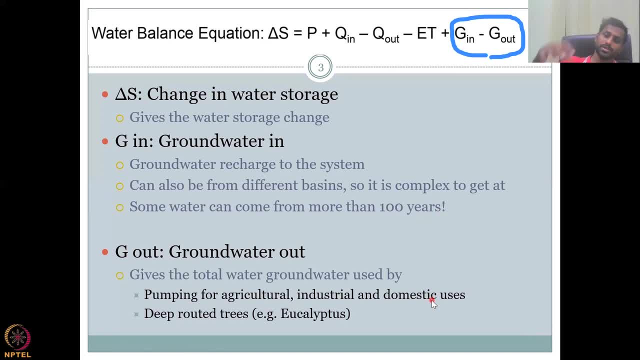 it is the total water used by pumping for agriculture, What happens in an industrial season? industrial and domestic uses. So what happens is that you have a pump and you take it out and that is discharged, because you are taking out the water for agriculture, industrial and domestic use. The other is natural. 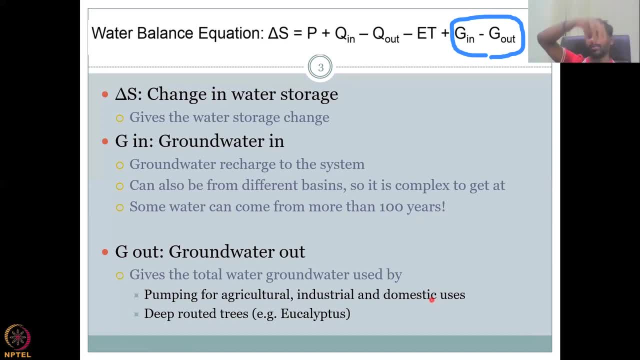 where you have deep rooted trees like eucalyptus and plants and other things which take water out, That is also kind of a discharge, but it goes into evapotranspiration. So So there is some part of double calculation in these. 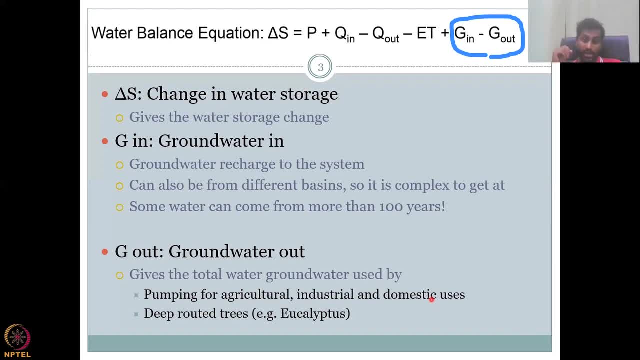 So it's better to say: ET is the water taken out by plants. However, when you pull the water out by trees, some water is raised up in the soil and it discharges out okay, So not all water is going to be taken by plants. 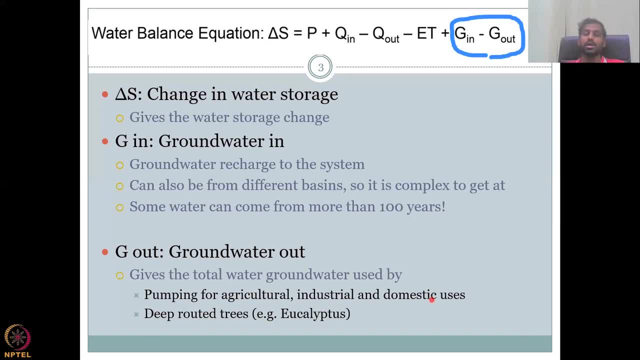 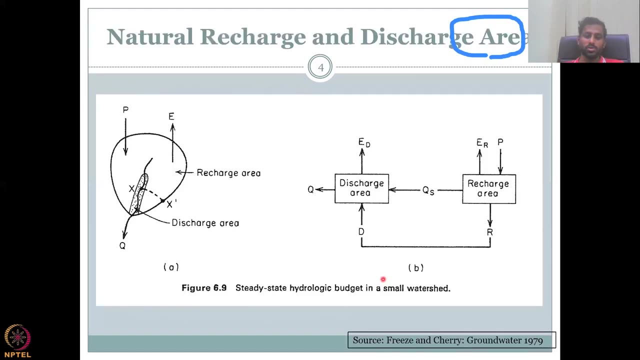 So that is the small component in groundwater discharge. But, most importantly, groundwater discharge happens naturally, as shown in the previous water cycle, by just seepage. It goes and joins the ocean, it goes and joins the rivers, etc. So let's look at the area to give an idea of how it looks like in terms of a basin. 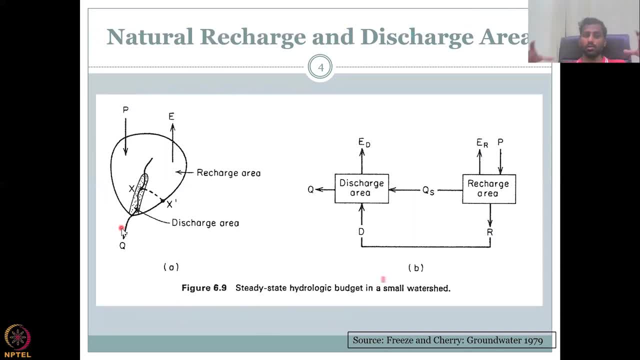 So you have a basin right And assuming that the water recharge is happening within the basin, just this basin, okay. So you have a basin boundary and you have, as the previous water balance equation I showed, you have precipitation coming in and evapotranspiration going out. 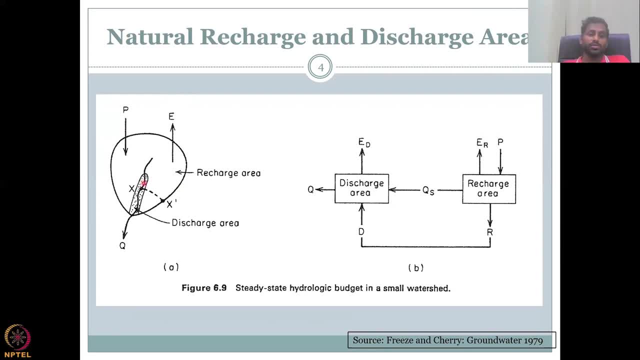 Here it is called as just one equation. Then you have Q out, which is your surface water going out. There is no Q in, because it is a basin closed for the water to come in. What you see here is there is a recharge area. 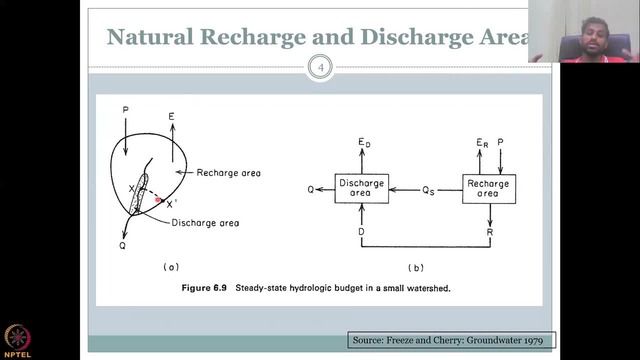 So when precipitation is falling on a particular area, all this area is contributing to recharge. So this is the area for recharge, Whereas for discharge it doesn't just discharge here because there's no elevation gradient or a water body that the groundwater wants to flow into, because groundwater flows from. 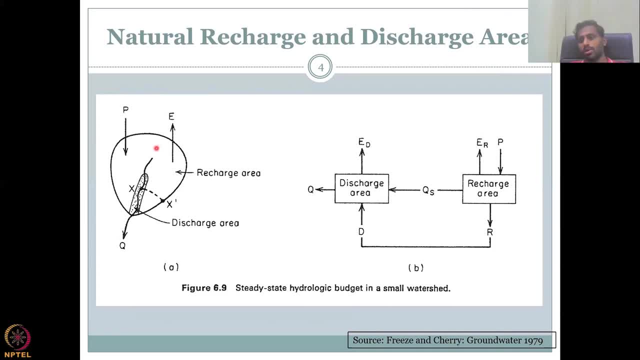 high potential to low potential. So here there's no water body that flows like that. What happens is along the channel, because the channel is already in a lower elevation and the groundwater potential is high in the groundwater, low in the water. So this is the area for recharge. 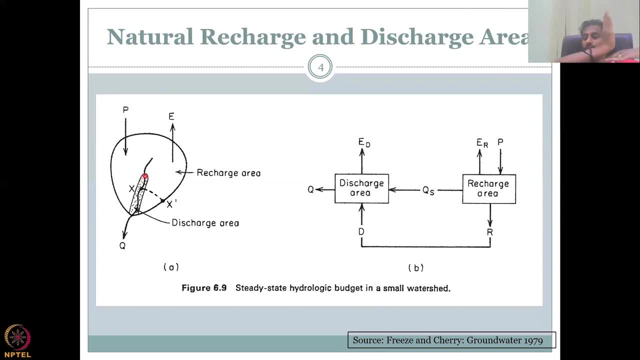 So this is the area for recharge. So in the stream the water would discharge out, So it will move like this and come out into the river And that is what this area is called. The dotted area is called the discharge area. Okay, 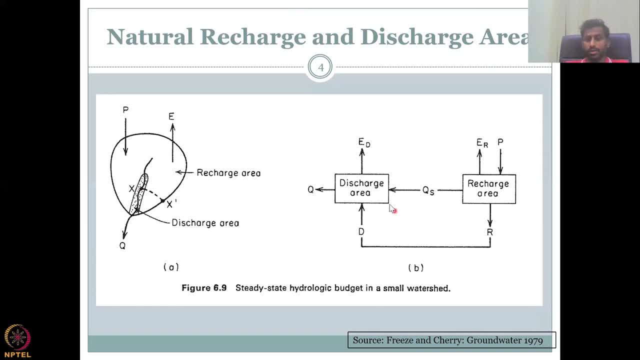 And look at the discharge area, You also have some evaporation along the discharge area and transpiration, Whereas all the precipitation is. it's very much less here, because already discharge is happening and precipitation will still fall on this area. Some recharge, but all the recharge would just come out as discharge. 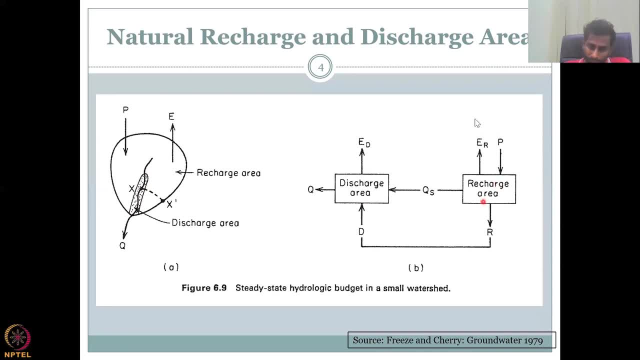 Okay, So in a recharge area precipitation is happening, Your evapotranspiration is happening and there is a recharge into the discharge area. So recharge and then recharge. water goes and discharges out of the discharge area. So this clearly explains the steady state hydrological budget in a small watershed. 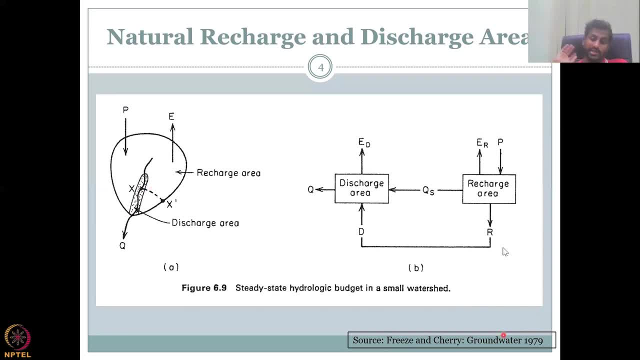 Where in, Q in is equal to Q out and it doesn't change. Okay, So, most important, what we need to understand here is the recharge area and discharge area can be within the same basin. However, they are differentiated because of the function and the function, as in how precipitation. 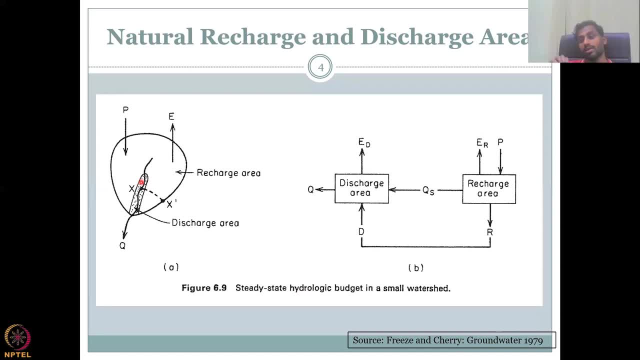 comes in how recharge happens and what is the area for discharge. So with this we can see that the discharge area is within the same basin. So with this understanding, we have a bigger groundwater recharge area compared to discharge area. Most, in most cases, the recharge area is bigger than the groundwater discharge area. 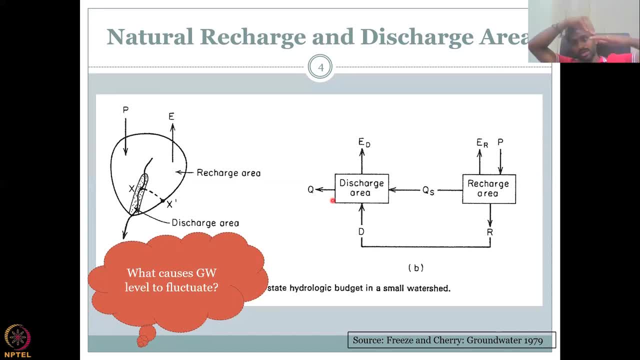 how groundwater comes out. So we know that when recharge happens, your storage changes. it goes up. Similarly, when you pull out water or water goes out of the system, the level goes down. So there is a fluctuation in the groundwater level. 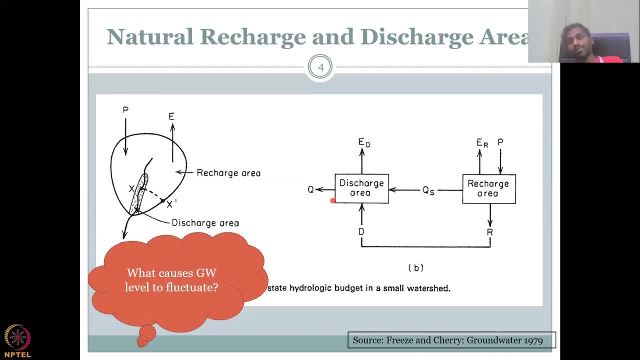 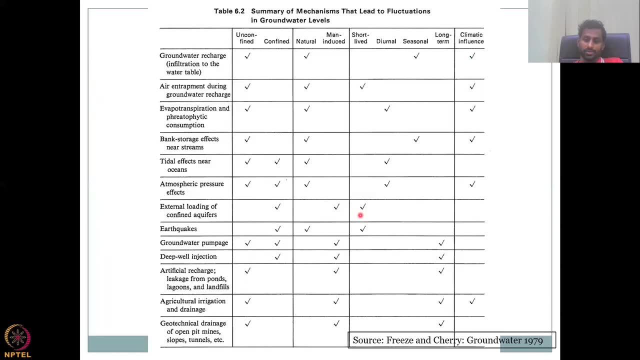 It is important. It is important to understand why these fluctuations happen. So let's look at a particular study from the freeze and cherry groundwater book, where they look at how these important mechanisms that lead to fluctuations in the groundwater- fluctuation means the water level fluctuates. 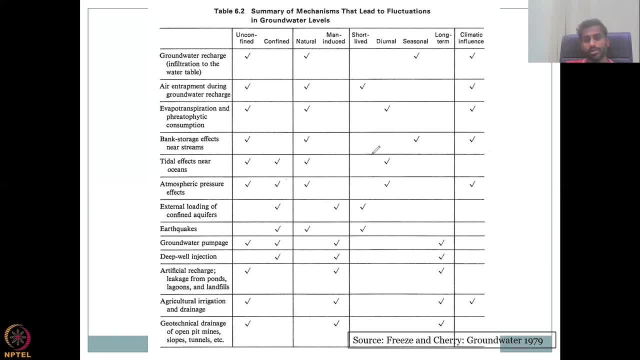 Just to draw a small thing. What do you mean when you- Because this term would be coming often in your books and stuff for groundwater. So this is your level. Okay, The initial level. The level can go up here or down here, based on if it is recharge, which is this one or? 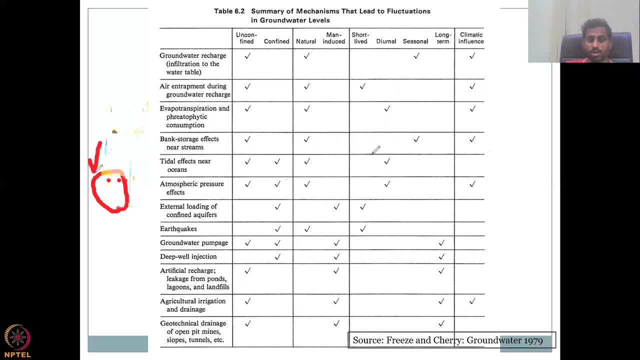 discharge, which is this one. So discharge is lowering of groundwater table because you're pulling water out, whereas recharge is raising of the water, Recharging of the water table because you're recharging water. So this is your new water level. I hope this is clear because it is important to understand the following notations. 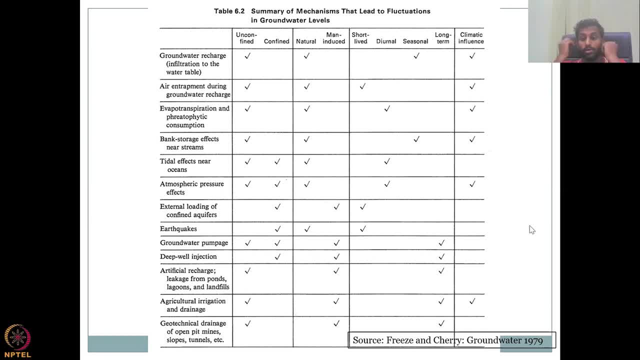 Let's go one by one, and we know what is the difference between unconfined and confined aquifers. We know what is natural and man-induced. Natural is it happens naturally in the ecosystem, whereas man-induced is the human interface is pushing that phenomena to happen. 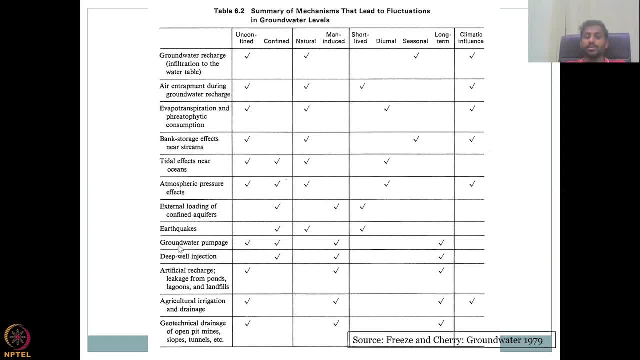 So what do you see on? your first column is your phenomenon process, And then the next set of column is whether the aquifer is unconfined or confined. Moving on, we have a next column, which is natural or man-induced, to show what is a key. 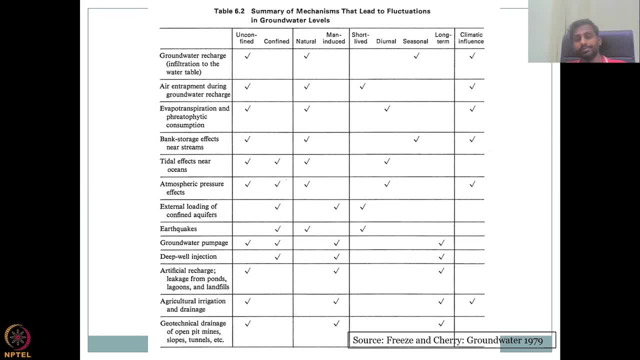 process driver for this phenomenon. Then the next is your duration. Is it short-lived? Diurnal means mostly daily, Seasonal, you have a couple of months or long-term, And then you have climatic influences. The climatic influences could be natural or man-induced. 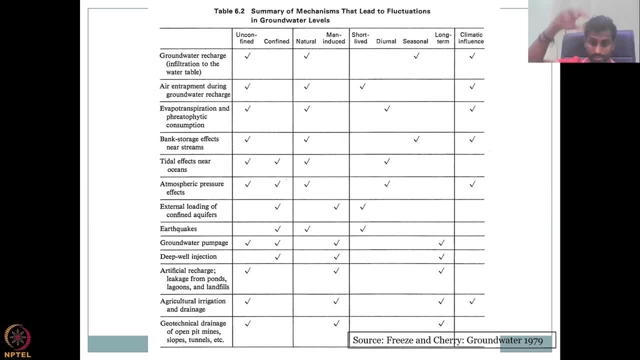 Let's not get into that Here. this climate, how the climate can induce it. So let's look at the most important Common processes that result in the fluctuation of the groundwater table or level. The first one is groundwater recharge infiltration to water table. 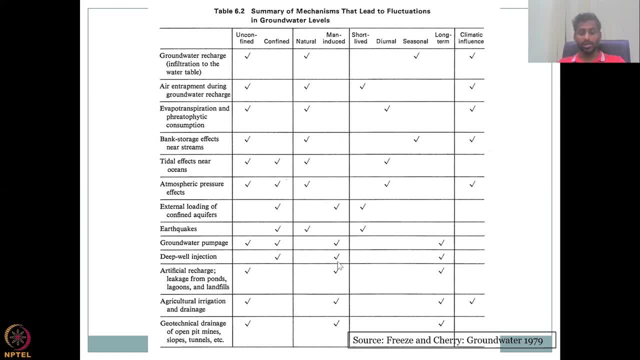 So, as I said, we do have groundwater recharge happening. Let's take this as the land and then you have water coming in right. So let's change the. The first one is groundwater recharge happening, infiltrating into the water table- And this is your water table, for example. 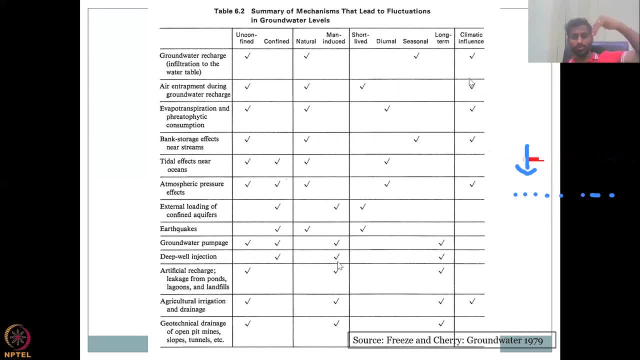 So the first process just documents the slow movement of infiltration and later percolation into the groundwater table. It can happen only in the unconfined aquifer. Why? Because let me also draw the unconfined and confined aquifer. So 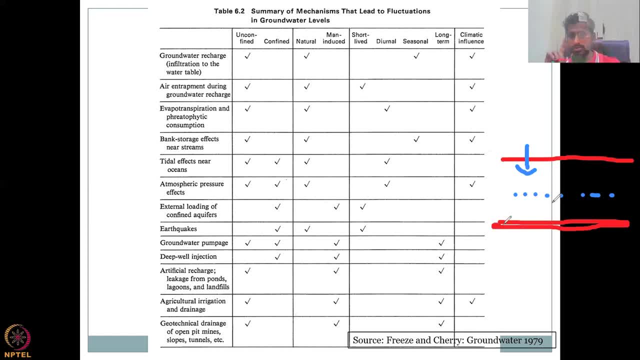 This is the second layer which has a thick, impervious surface, and this is your one and two. Okay, And this is your bottom layer, the drop rate. So let's move on the first groundwater table. The groundwater recharge moves through from rainfall or some other water like irrigation. 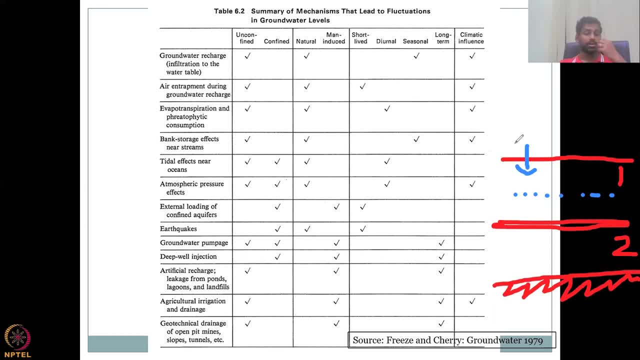 You have a tank which is leading into a canal irrigation or just water flow. Water can irrigate, like gardening and et cetera, right, So that water can infiltrate into the ground and raise the water level. That can happen only in the unconfined layer, because the unconfined layer is open to infiltration. 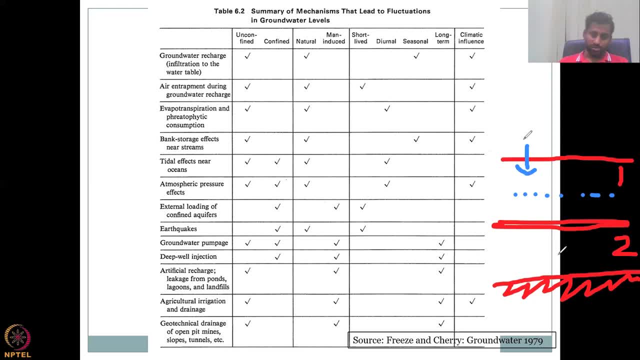 Whereas the confined layer is not going to change. So there is no tick mark. There's only a tick mark in the unconfined layer. Is it natural or man induced? Mostly So, yeah, There could be some man induced, like you can push water through focused infiltration processes. 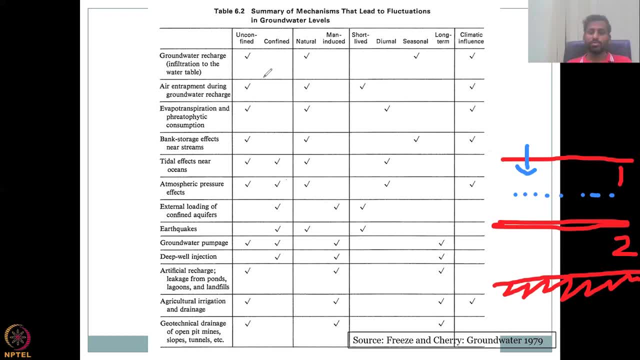 but in general, in general, it is nature, natural based process. because of soil, because of rainfall, because of gravity, you have infiltration and that actually raises your water table. Okay, Let me put a small tick here, just to show that you can have groundwater recharge. 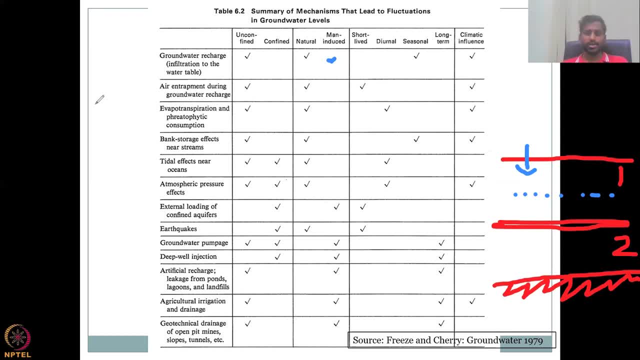 Recharge networks, surface ponds- okay, Farm ponds- etc. That we saw. we will be seeing. Everything is there. Is it short lived, diurnal or seasonal? Mostly it is seasonal because the rainfall happens not very short lived, It is not daily. 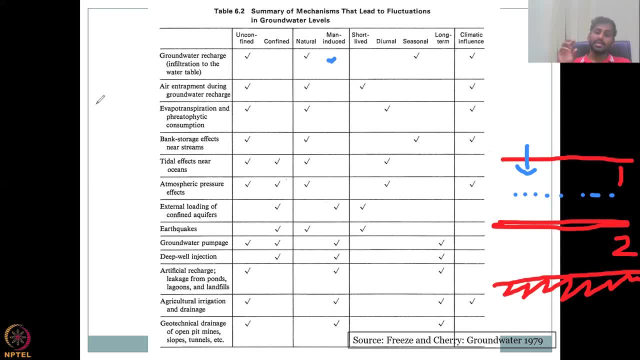 Just within a day it will change. It is a seasonal pattern. Okay, Not long-term, because every season you do have recharge. Is it influenced by climatic factors? Yes, Because when climate exists, it is a seasonal pattern, So there is a season. 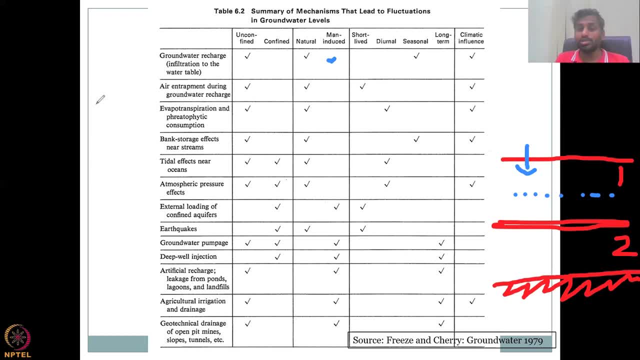 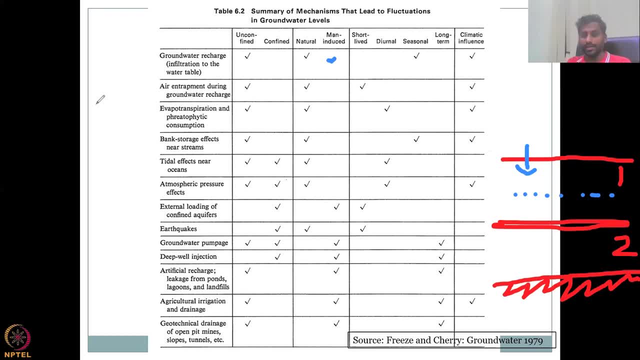 It is seasonal. Is it influenced by climatic factors? Yes, because when climate extremes happen, for example your flood, there'll be more rainfall happening and stagnation of water, so water can recharge What happens in the drought, which is also climate extreme. 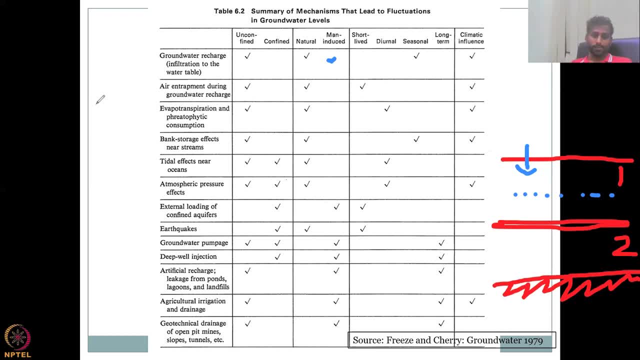 There is no water. When there's no water, there's no recharge, Then what happens is you have extreme events also and a slow tapering event which is you're increasing, increasing rainfall. not a flood, I'm saying, but rainfall is increasing. 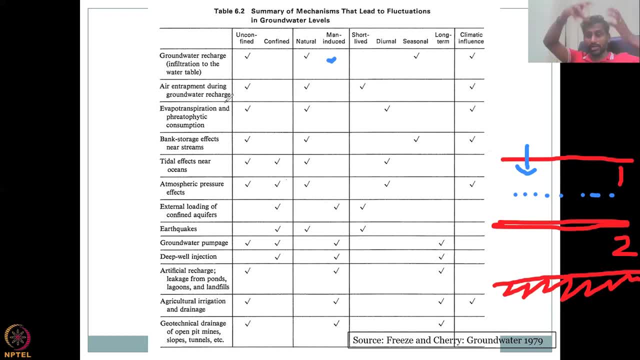 and your temperature is increasing. So when you have high temperature, water is less, so infiltration is less, because all the water will be evaporated. So all this is the first row which talks about groundwater recharge through infiltration, which infects your fluctuation in the water table. 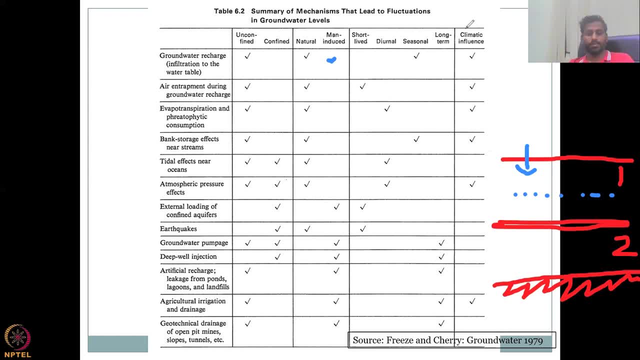 can happen through climatic factors. Moving on, the second one is air entrapment during groundwater recharge. So think that when groundwater is coming, your recharge is happening by one, the first process. okay. So when groundwater recharge is happening and we have to thank Fries and Cherry's book, 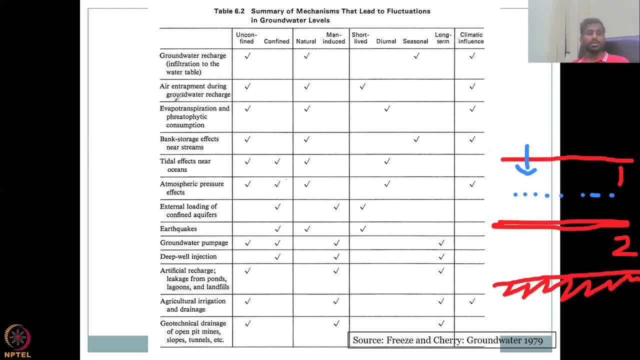 which has documented everything very meticulously. These constitute all the major processes for fluctuation, fluctuation of water table in the water cycle, and we can differentiate that as recharge and discharge. okay, So a big thanks to the book And we will look at the first thing. 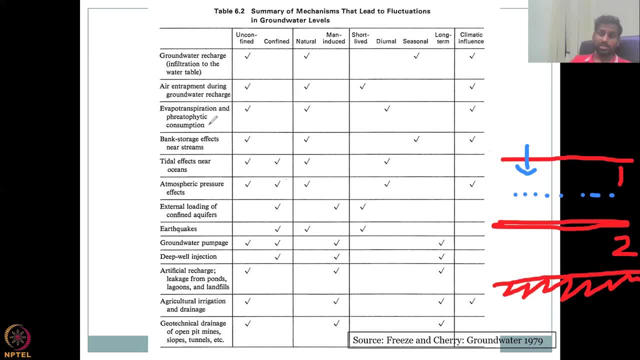 which is air entrapment during groundwater recharge from the recharge. So the first one was the recharge and then, while the recharge is happening, think about this: You have land Inside, you have soil with porous space and the space has air or water or none. okay, 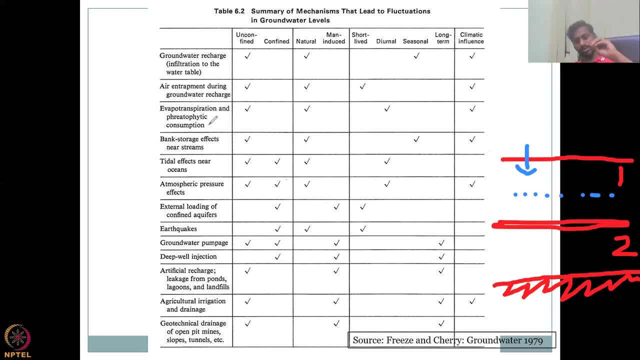 combination of both or not. Suppose the air is present in the porous space, So when water comes in, the air either has to be displaced. Okay, So the air sometimes get entraps during the groundwater recharge. How does that influence your water table? Basically, you have less water going into. the water table to have fluctuation, or the water bubble can go in to the water table and raise it until the bubble breaks. Okay, So that is only in the unconfined layer, Only in the top layer. it happens, It doesn't go in. It doesn't go in the confined layer because air moving that far, it cannot, because by the time it moves into the small small pores and goes down, it's ripped into very small particles and it doesn't become a bubble kind of thing or entrapment. It is purely nature based, because water is being pushed by the groundwater. 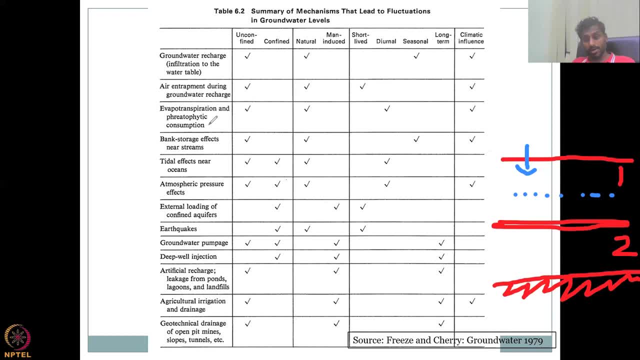 water recharge And it is very short lived. In fact, it is one of the least important processes for groundwater fluctuation. However, it fluctuates And it is also influenced by climatic factors, Because if it's a very hot surface, then all the water is taken out full. 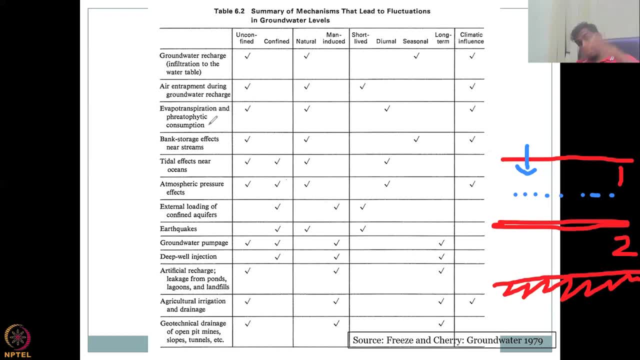 of air is in the soil And then, when the rainfall happens, suddenly, before the air can escape, a big rainfall pushes the air bubble inside. So the air bubble gets trapped, But what it is is the entire process of the fluctuation. the fluctuation of the water table is just 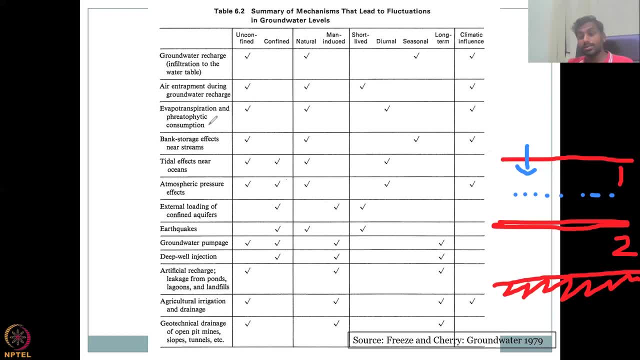 short lived. It just blip and then comes down. This is important to understand while you're in the field, because a lot of these field instruments will throw this error at you, sudden error, And you'd be like, oh, there's no rainfall, or that was not big rainfall. 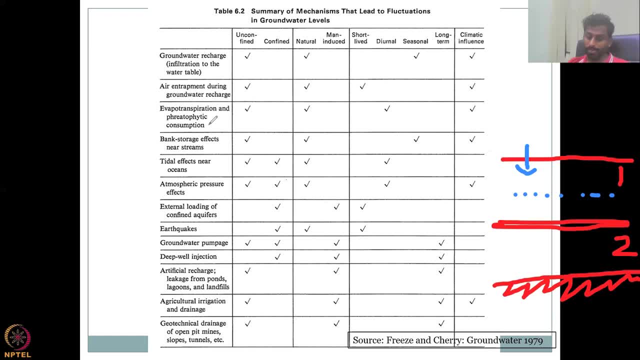 Or why is it short lived? Suddenly there's a blip and comes down, And that is explained by air entrapment. And many, many other instruments also have this, like, for example, the discharge measuring devices, water flow- Suddenly there is a eddy current or a water and droplet which is stuck in. 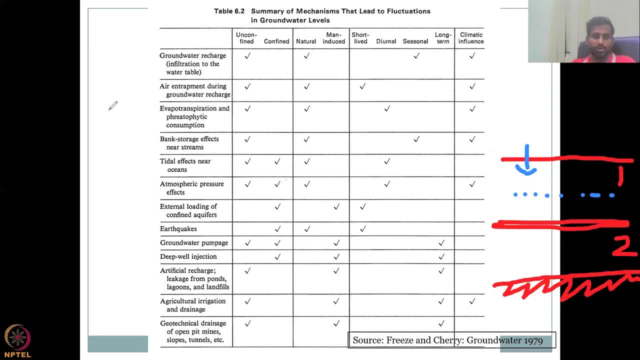 the machine. The next one is evapotranspiration and phryotrophitic consumption. Let's just keep it as plant consumption. So what happens in the unconfined layer? Again, we are talking about plants and trees that are accessing water only from this layer. So when they pull the water out, eventually, your groundwater table goes up and down. It goes up slightly when the water comes in because of the pull, but most importantly, water is pushed down. The water level is coming down because more water is being sucked out. So this happens also as a phenomena in the unconfined. 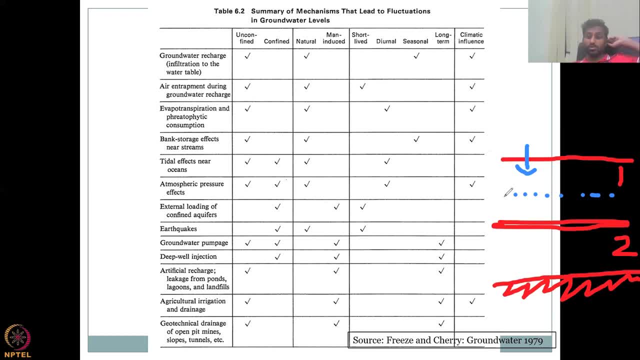 aquifer. It is by natural based system, because plants are nature based systems. It is not short lived, It is diurnal. Why diurnal? Because the growing cycle is also serial. diurnal right Because the plant sucks the water only in the daytime when transpiration happens After. 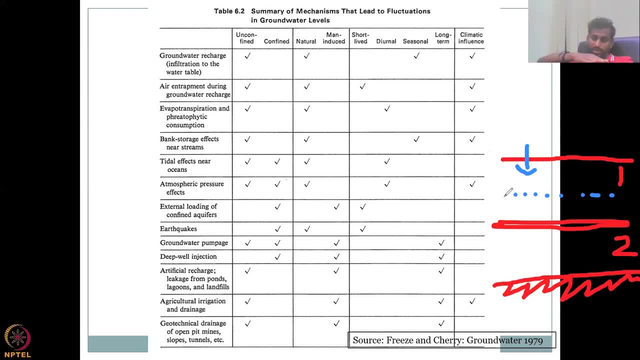 that it shuts down. So suddenly you see a groundwater plummet and then it slowly comes up, comes down, goes up, comes down, goes up, And this science is called the natural sinusoidal nature of the water table mimics your water use of the plant, When the plant 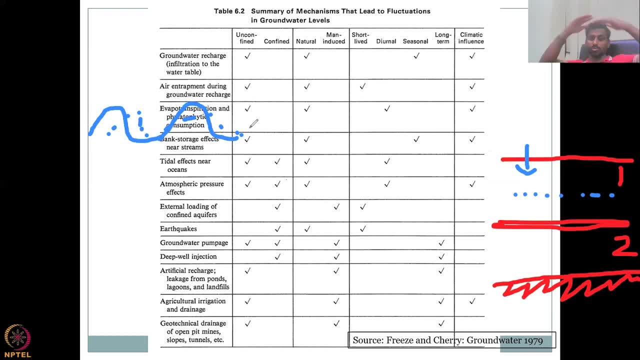 takes more water, it goes down. And when plant shuts down, sun shuts down, there's no photosynthetic reaction taking place. then the water recharges up, Moving on. then it is also influenced by climatic factors, because when there is a different 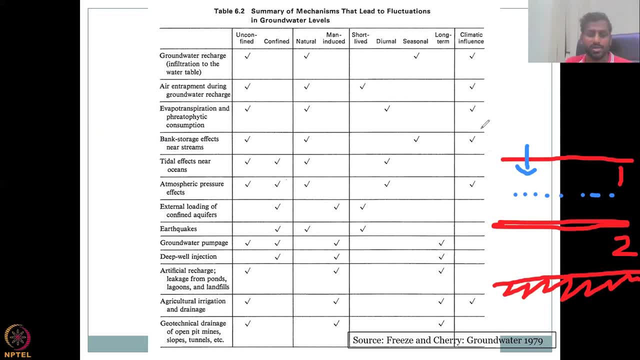 climatic pressure on the plant. the plant water consumption is different. Bank storage affects near streams. So, for example, you have a stream, you have a river flow Near the river. there could be some water stored because of the flood. Okay, a flood, big flood is coming and the bank. 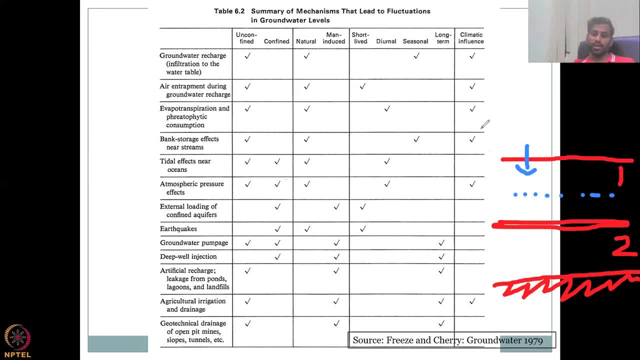 is full of water, That can also influence your unconfined aquifer, the first layer in the aquifer, because the water can raise based on the bank water storage amount. It is purely a natural based system and it is seasonal because your river will have water. only during seasons When there is no water flow. in the season there is no water in the river and it is dry, So the water table is down. Once water flows from your river channel, from your bank water, water will come down into the groundwater aquifer and recharge. 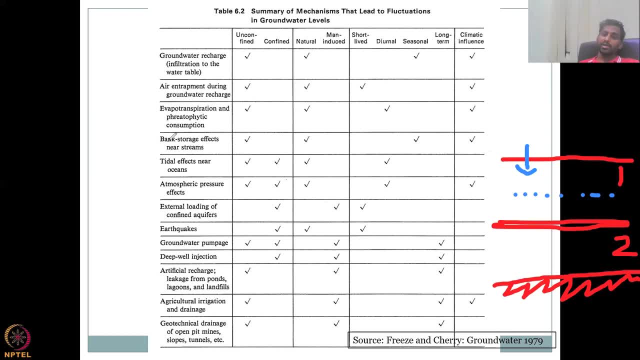 your aquifer. It is also influenced by climatic factors- big mud and sand- So it is also influenced by the climate factors. So the water is running down the bank and it is also influenced by the water storage amount Because, based on the climatic factors, you have water coming into the river. Because if there's a big rain, a lot of water will come in the river And that water will flow as flood and the flood will induce recharge Tidal effects near oceans similarly. Similarly, you have big waves, big tides that will come and hit the coast. And that happens in a cyclic pattern. also, During certain periods of the month you have a bigger tide and then small tide. big tide, small tide. So when this big tide comes, more water reaches the shore and that water can recharge. So that is also an unconfined aquifer effect. But because the volume of water is too big and it pushes the water comes in a big force, it can also impact your unconfined aquifer. So both unconfined and confined Unconfined aquifer can be influenced by this tidal effects. 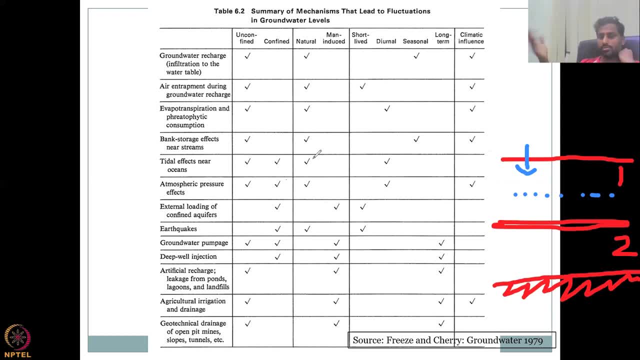 It is a purely nature-based system, even though man-induced climate change and other things can happen, And it is diurnal nature. If you go to the beach, you'll see that during the night the wave is high. During certain peaks of the month it is high. 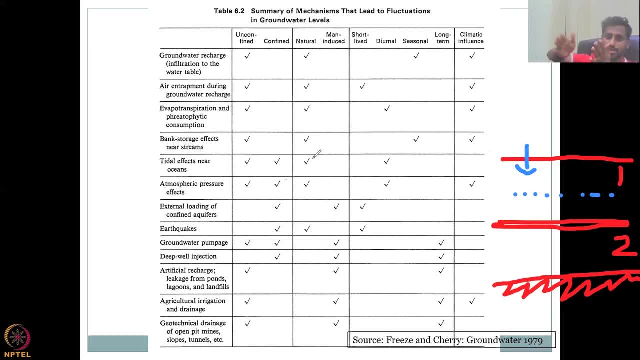 So it's not a seasonal. It is between the seasonal and diurnal. Diurnal is daily, Seasonal is a couple of months once. So you could see that The water recharged through tidal can happen in a nature-based system. It is diurnal daily. It happens because day and night, day and night, Okay, And it may or may not be influenced by climatic factors, Atmospheric pressure effects. So when the atmosphere pressure is different, water can come out, because water flows from high potential to low potential. 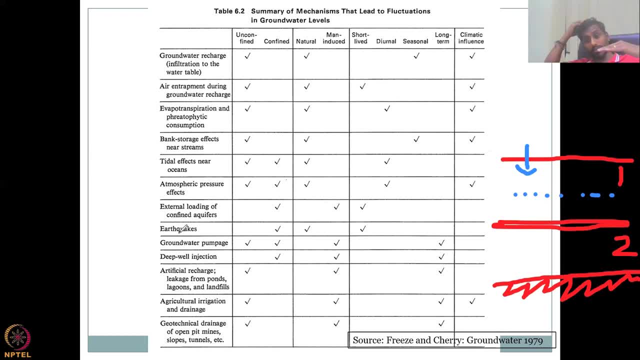 For example, outside the well, if the atmospheric pressure is low compared to high pressure of the water inside, then water flows from high pressure to low pressure. You have automatically flowing wells, which are called artisan wells. We saw this in the first couple of classes. Okay, And that is purely happening as a climate influence factor, because the climate changes your atmospheric pressure. It can happen from unconfined or confined aquifers, basically where your well is placed. Okay, And it can happen from that aspect also, And also it is a very natural based system because it can happen only from a deep well and because of the atmospheric pressure. 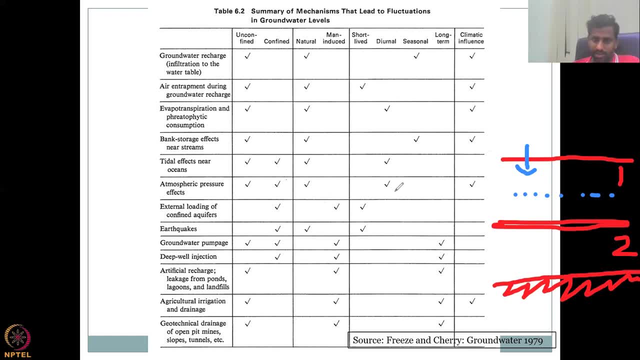 Humans cannot control the atmospheric pressure. It is diurnal in nature and can be influenced by climatic factors. Diurnal because every day, in some aspects, it can happen. External loading of confined aquifers. So you have unconfined. So you have unconfined. 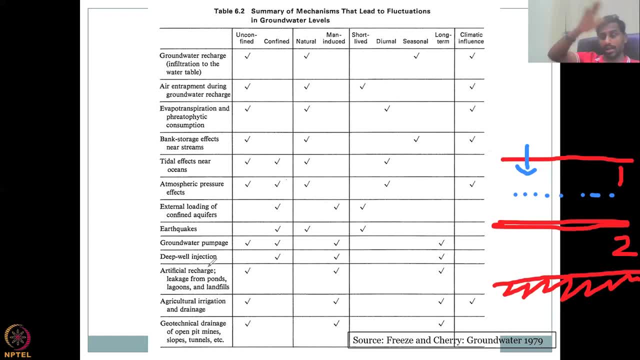 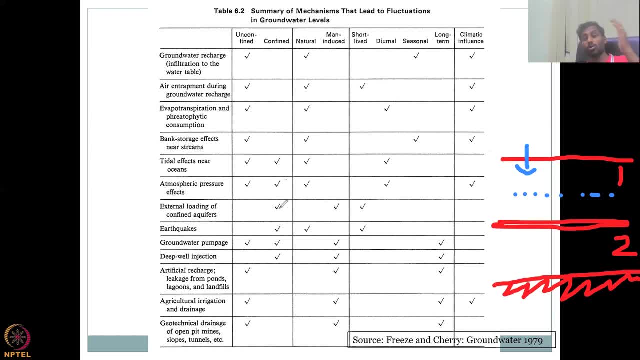 Okay, Only confined aquifer layer is there, And as external loading happens, it can happen, naturally, but only once. It's not a big thing to record, But it is a man-induced part, So that happens in a couple of times. 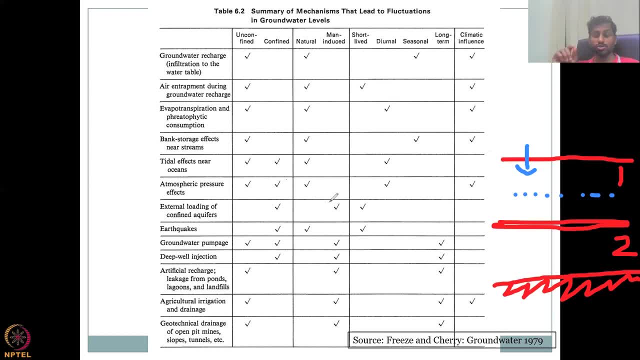 Then it is because of human-induced. It is very, very. It is very, very short-lived. Suddenly you put some loading. For example, you bring a big couple of tons of cement and blocks and put it on top of the aquifer. 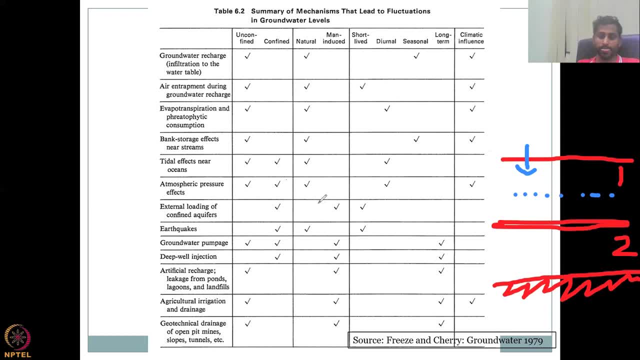 It just pushes your aquifer and suddenly you see a jump, fluctuation. There's no climate and other things- Earthquakes. Earthquakes are the process in which the plates very, very deep near the bedrock- near this area I'm saying, where the rocks and other things would move. So when they move, the water table Also fluctuates because of: suddenly, if there's a crack, then this water will flow down. Water will come down, or if there's a crack and water flows out of the system, then this water level will go up. 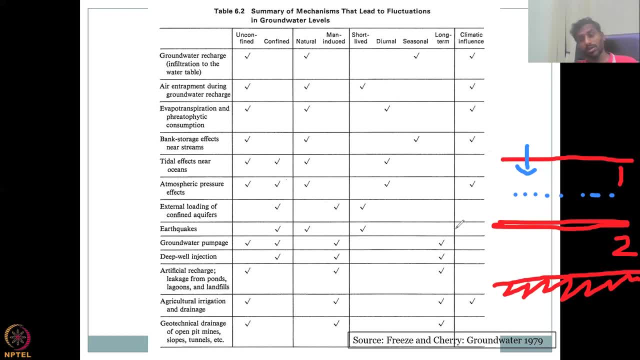 Right. So these define the water level fluctuations because of an earthquake, Um and it happens only in the confined aquifer because of the depth. It is a nature-based um process and is very short-lived: just a couple of minutes, That's it. 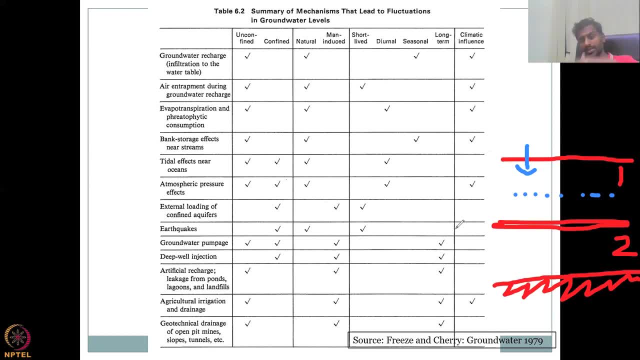 It's not going to be every day It's going to shake, or every season is going to shake- earthquake. Groundwater pump is the most important aspect in groundwater fluctuation. Pumpage can happen from unconfined or confined aquifer, based on where you're putting the pump. 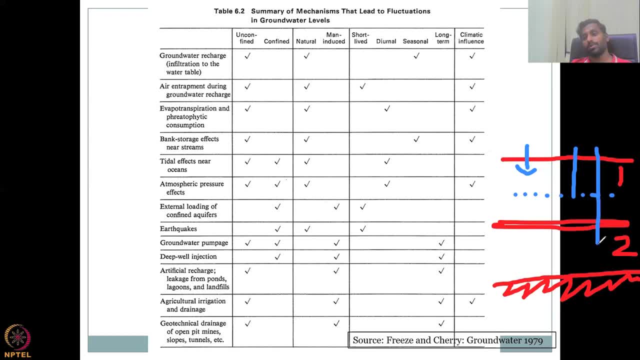 You can have one pump in the uh- unconfined and one pump in the confined So you can pull the water out. It can change And it is a human based process because you are the one who's going to do it. 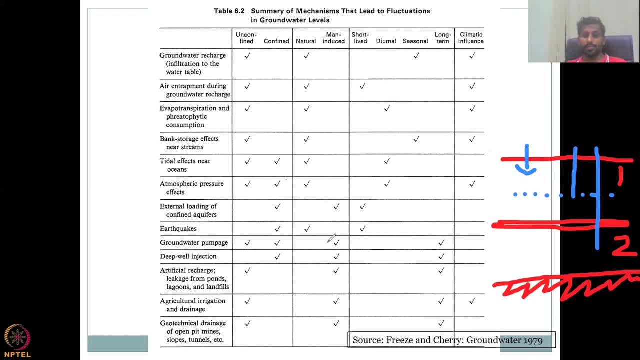 Okay, Okay, Okay Okay, You're the one who's going to control the pumps. It is um also long-term effect because once you pull it, the water still table will take long time to stabilize. It's not going to uh, fluctuate and then stay there. 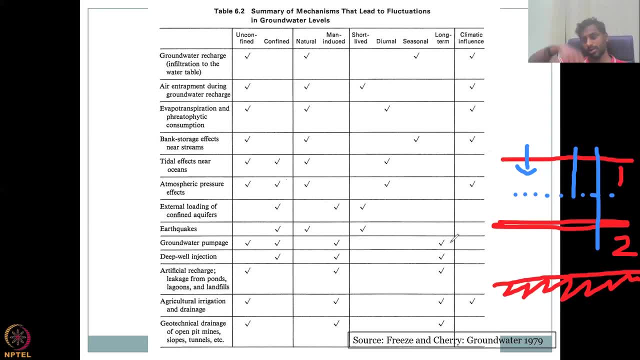 It just takes slowly, slowly, slowly or easily You'll pull it out, So suddenly the water table will fluctuate down, but then the recharge happens very slowly. Okay, Deep well injection: This is also a human induced process and injection. 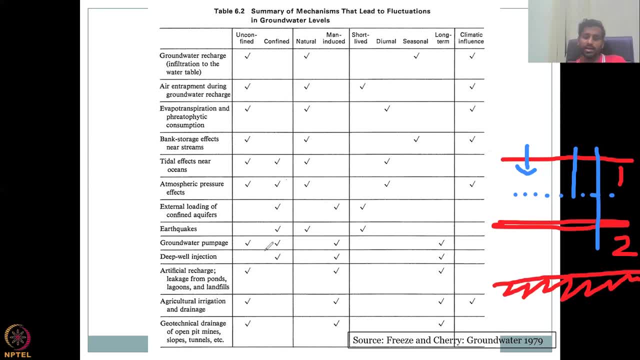 You put in water, okay, and it is in the confined aquifer, So the confined aquifer is here. You put in some water for some process, fracturing, or you want to uh put in a pollutant water, like some people do- uh, very bad, you know, for polluting the environment, or you want. 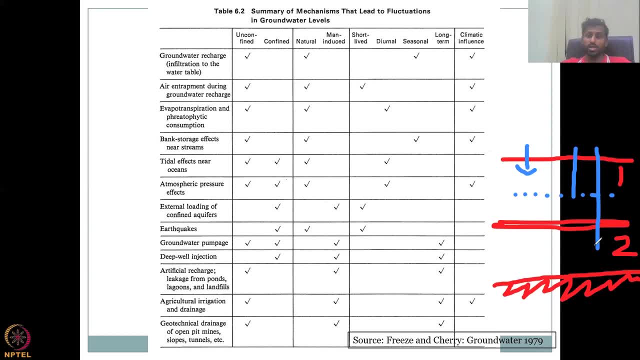 to actually recharge or keep it in the ground so that you can use it during the later season, like UTF-5 project I mentioned. So this deep well injection is It is based on a reverse of the pump. Instead of pumping out, you're pushing water in using energy. 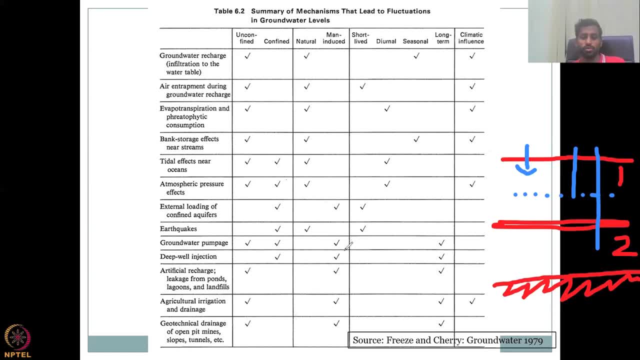 Uh, it is a confined uh aquifer process, manmade, human uh influenced, and it is also a long-term similar. like you're pumping, It is also long-term artificial recharge leakage from ponds, lagoons um and other landfills. 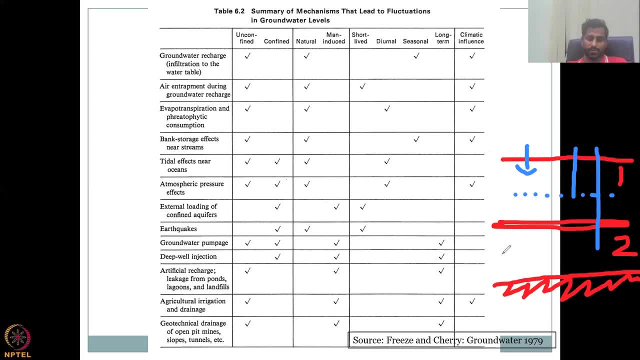 It is where you create or you induce more recharge, And that happens mostly in the unconfined layer, the top layer, Because that is where most of these small structures would push water in, not to the deep aquifer. Okay, Uh, it is uh manmade, because it is artificial. just know this word. 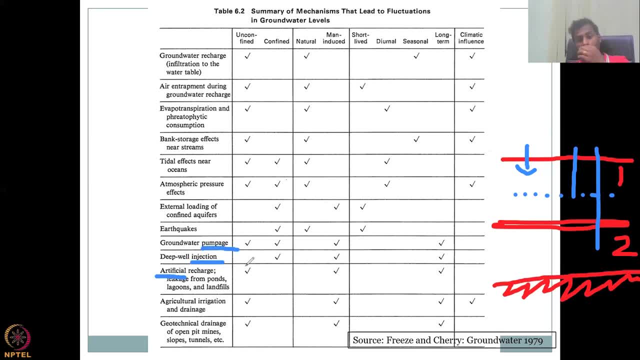 It is artificial injection, pumpage. all these are caused by humans, So that is defines if it is human or natural. It is also long-term. Okay, It is not a very short-term process because it takes time for it to go in and stabilizes. 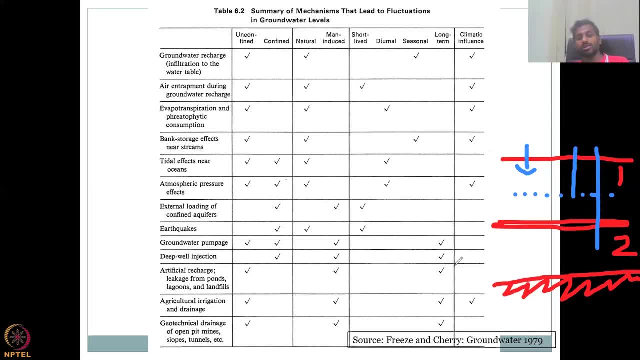 the water level. Okay, Then we come to agricultural irrigation and drainage. So agriculture itself is a manmade or human influence process. It is happening only in the unconfined region, because agricultural irrigation, not other, that's pumping, Okay, Uh, I think it's irrigation. 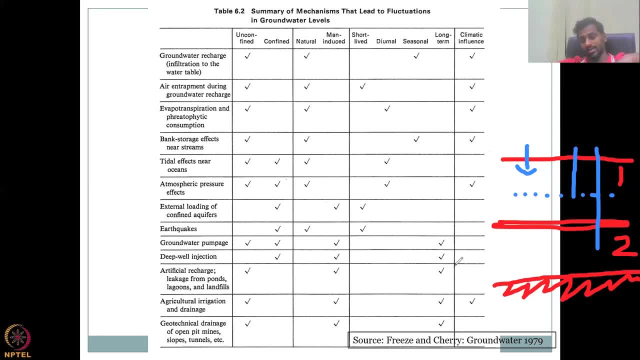 You're going to put water on the surface and water recharges. It recharges only in the unconfined layer, because the roots are only here. The plant roots will only grow to here. It doesn't grow much. Right, It is a manmade, because agriculture is not a natural process or a standard things a. 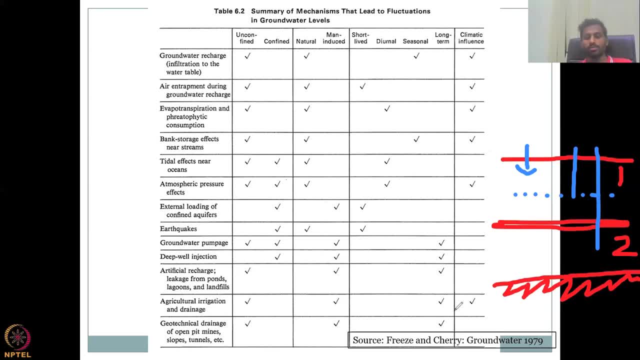 natural process And then it is also a long-term, like pumpage et cetera. whatever it is human induced, it is long-term impact. It can be influenced by climate because the climate factors influence how the plant grows: Geotechnical drainage of open pit by mines, slopes, tunnels, et cetera. 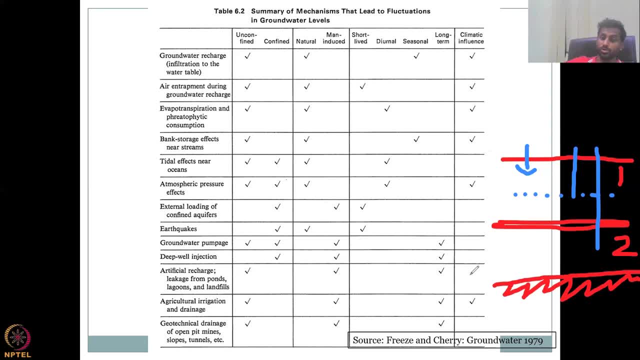 Uh, this is the geo technical, Okay, So the geotechnical drainage, because you push water into, uh, these kinds of, um, uh, pits, mines, et cetera. So mine, mine, when you have a mine where they collect the ores and stuff, uh, they. 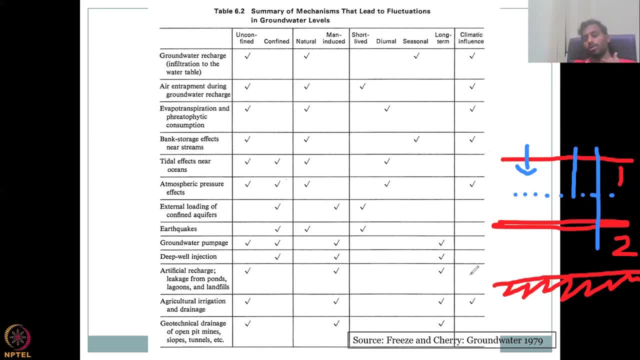 have a specific space where they can put all this, uh dump all this water, uh slopes, tunnels. Also, when they cut, there's some space where the water goes in. Okay, So suddenly you see, uh an influence on the confined, unconfined aquifer. 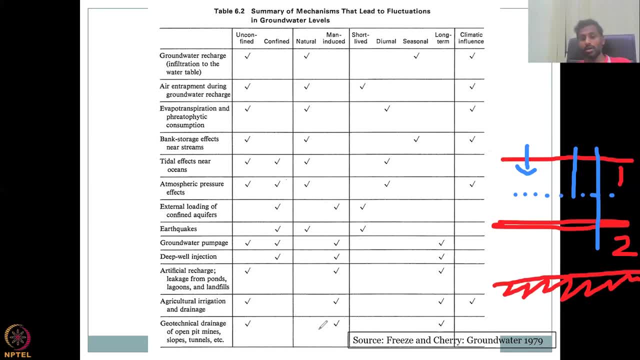 The unconfined aquifer changes the level. It is a human um induced um process. It is also long-term. So, uh, there is no climatic factors. So what does it take home here? There's multiple things that can change the water level, either by recharge or by discharge. 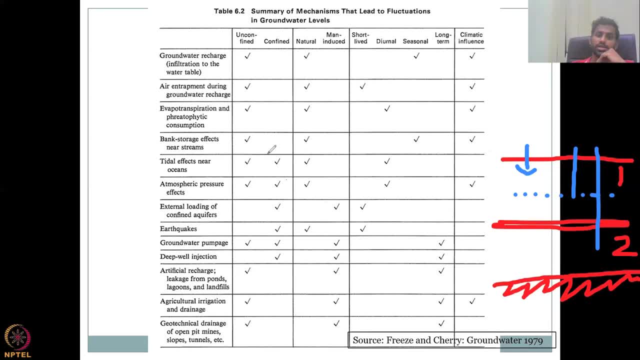 taking out the water or putting in the water. What you see is the nature based uh processes are either seasonal, short-term or diurnal, Whereas the human based processes are long-term. So when you disturb a system and it takes long-term to stabilize, that is not sustainable. 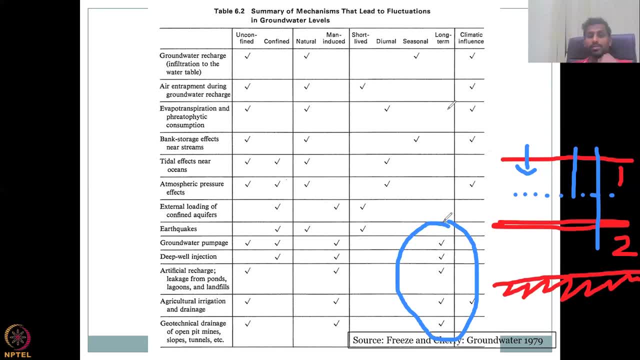 You cannot do it continuously. Okay, For example, the man storage can happen continuously, because every season the water comes. it's fine Uh. however, your pumping injection, artificial recharge, agriculture irrigation, which is also artificial, um uh plants and vegetation. 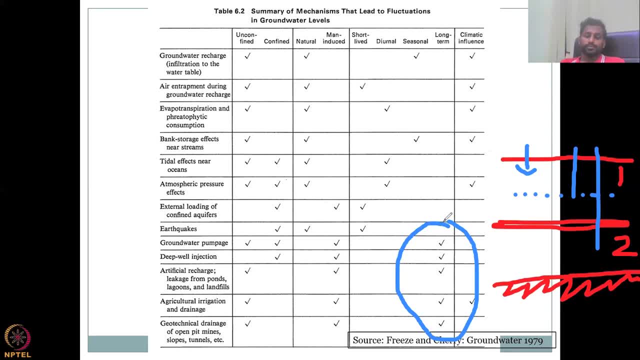 You're growing, not by natural process and geotechnical drainage. all this has an influence on the groundwater aquifer because you are pushing water or you're extracting water, And the more key uh driving home message, or the drive home message is these take time. 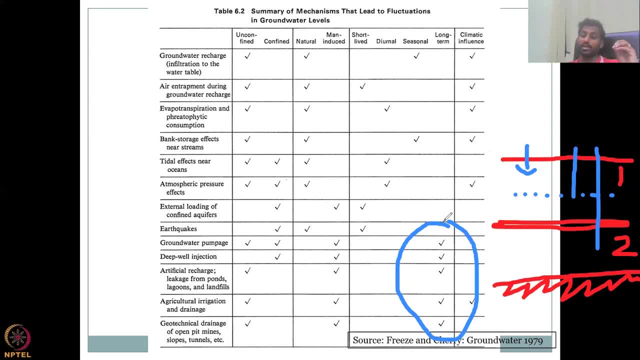 It is also influenced by climatic factors, but, most importantly, it takes a long time for the water to stabilize, the fluctuations to stabilize. So, And what is going to happen next? If I take too much water, the water level comes down um and before I know how much. 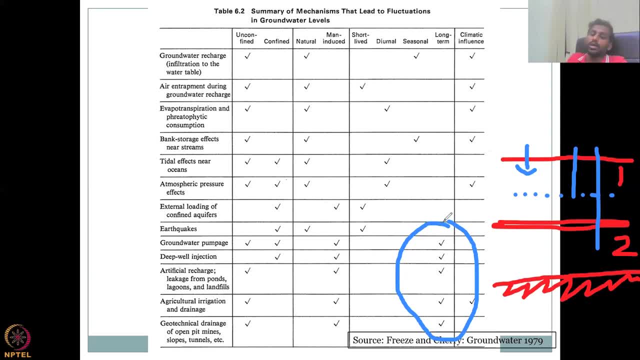 water is there. I can pump, but I can pump, And that is why the groundwater resources are very low in the country, especially India, where most of the groundwater is extracted. I hope these messages were clear to understand. um, you know all the um important uh. 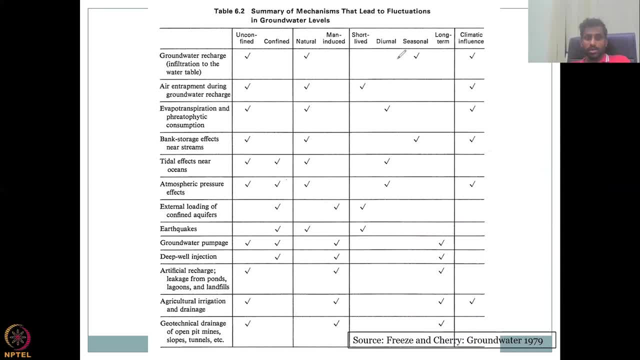 process through which fluctuations happen. I will See you in the next class, where we go on to discuss each one process, in particular because recharge is different than discharge. So we'll go on to see how recharge happens and how are they estimated. Same way, we'll go to discharge and see how discharge happens and how it is estimated. 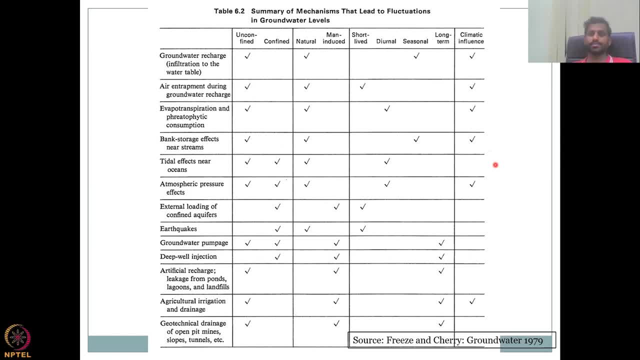 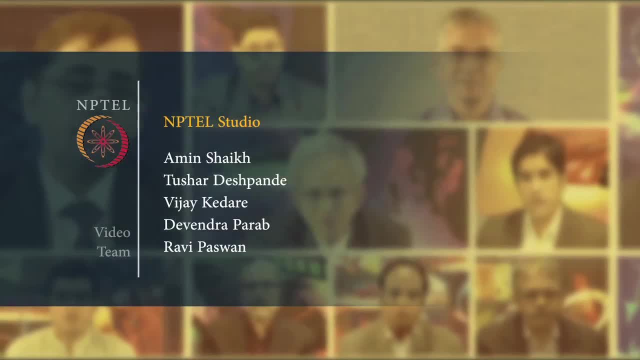 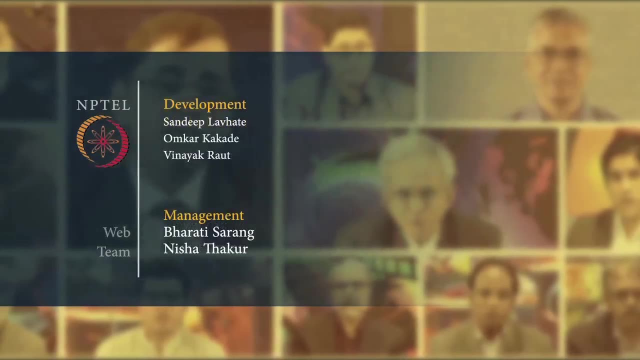 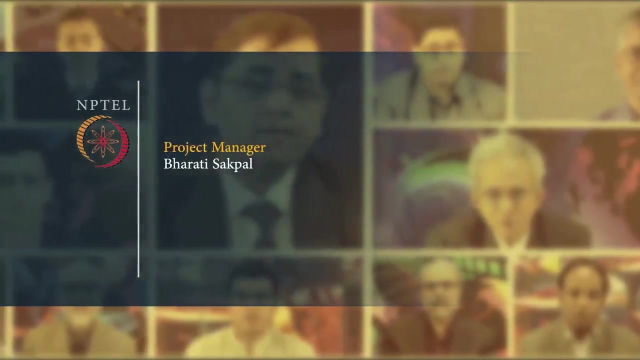 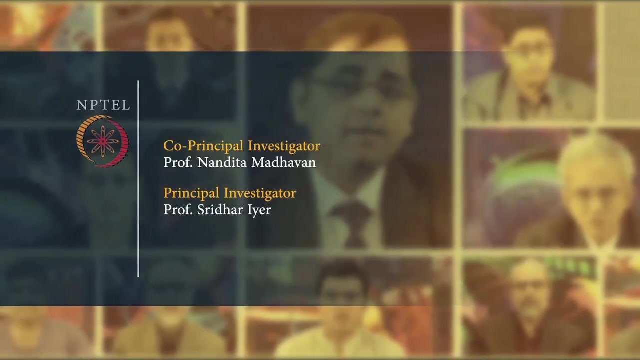 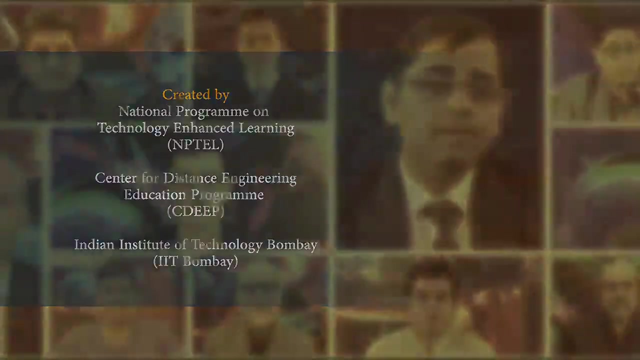 Thank you. I will see you in the next class. Thank you, Bye.